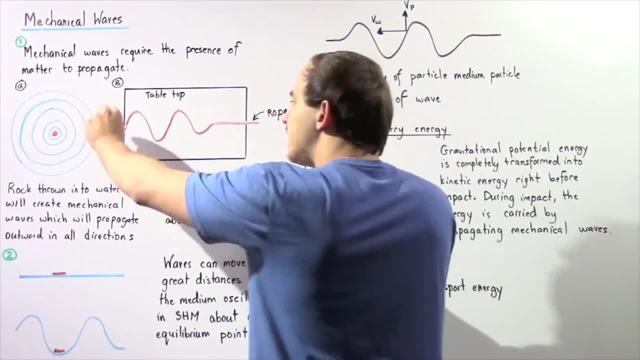 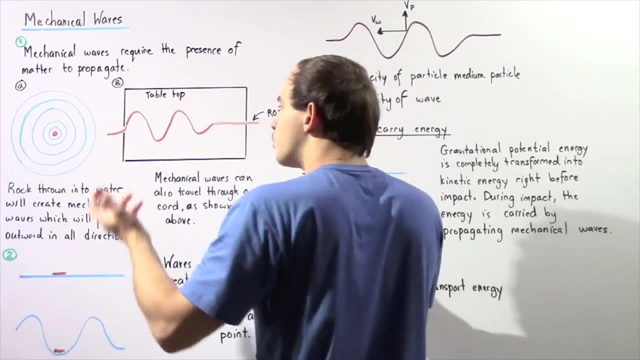 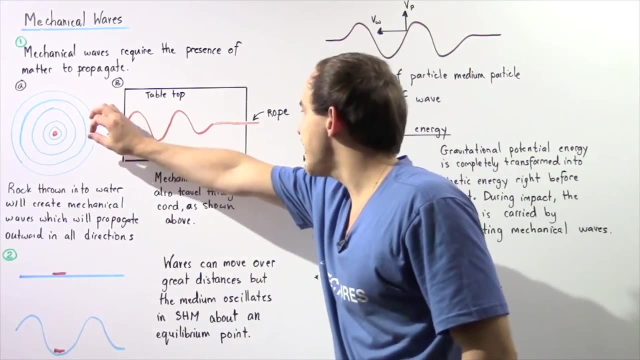 and we take the cord at one end and we oscillate it in the following manner. So that will create the movement of our hand, will create the following oscillation, Which will create a mechanical wave that will propagate in the following rope, So the medium in 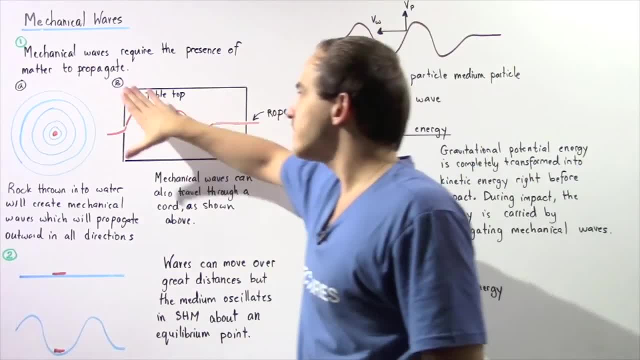 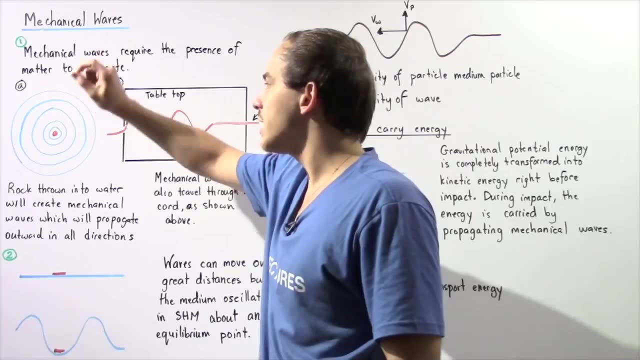 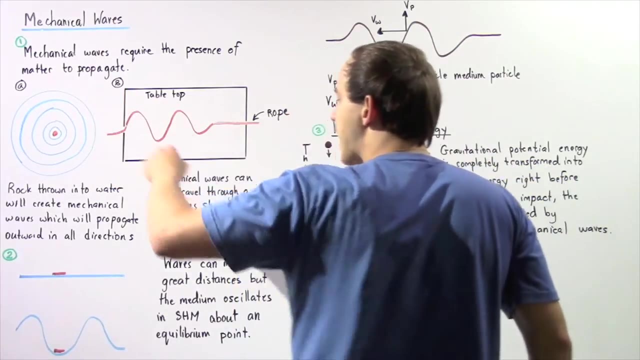 in example B is our rope. So we have the top to bottom view of our circular waves that are created by the impact between the rock and the water. And in part B, what creates the mechanical wave is the motion of our hand that forces the rope to propagate. 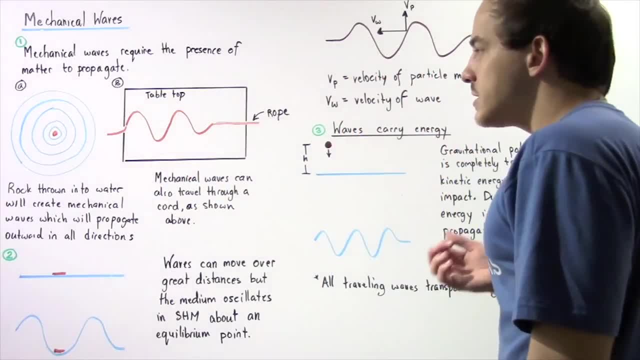 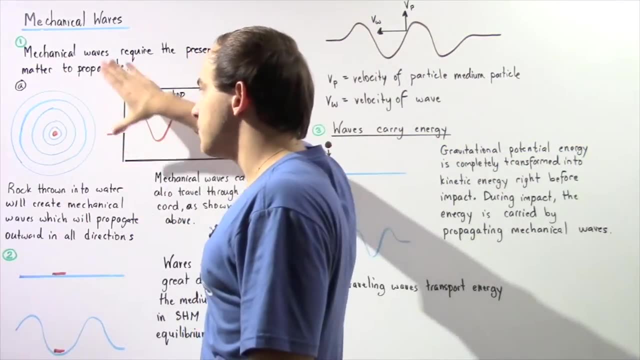 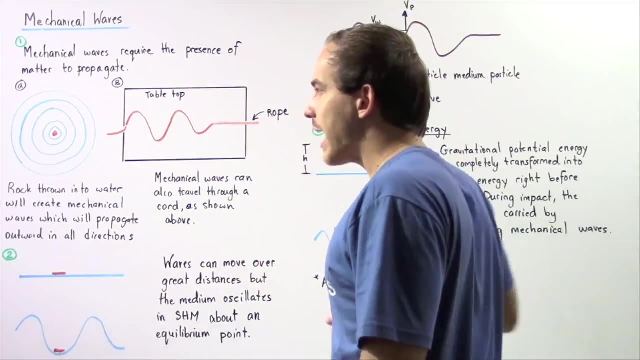 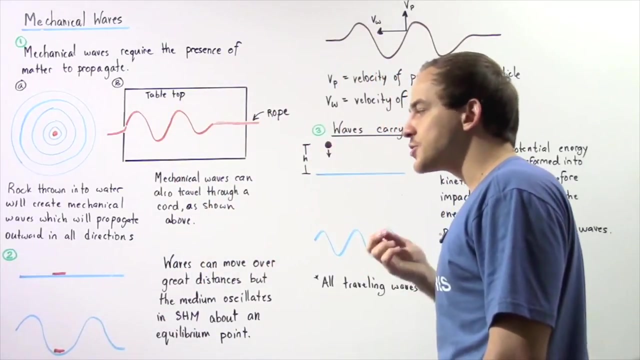 Now let's suppose that we want to examine the side view of example A. So this was the top to bottom view. Now let's examine the side view. So let's suppose, right before we let go of our object, the surface of the water is still, and on the surface of the water we have a certain floating object. So let's suppose that 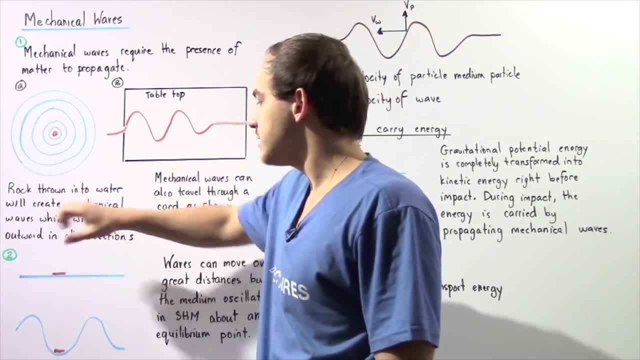 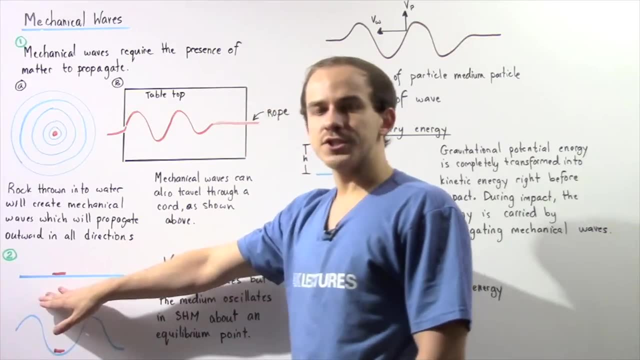 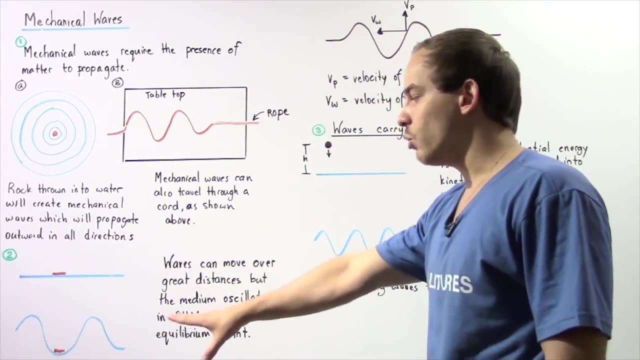 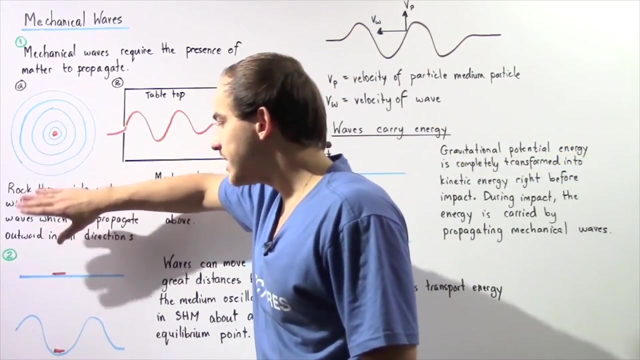 floating object is a leaf floating on top of our liquid. Now, what happens when the object actually hits the surface of the water? Well, when the object hits the surface of the water, the water begins to propagate in the following direction. Now I want to ask the following question: Does this object floating 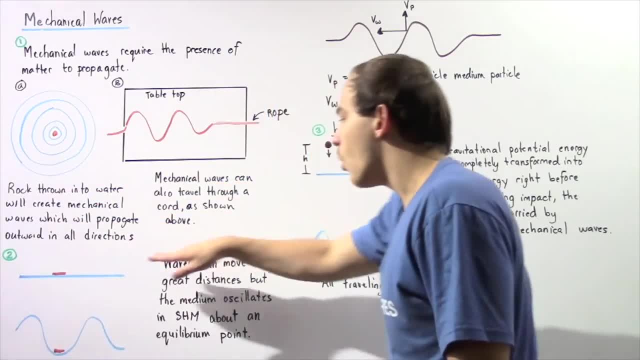 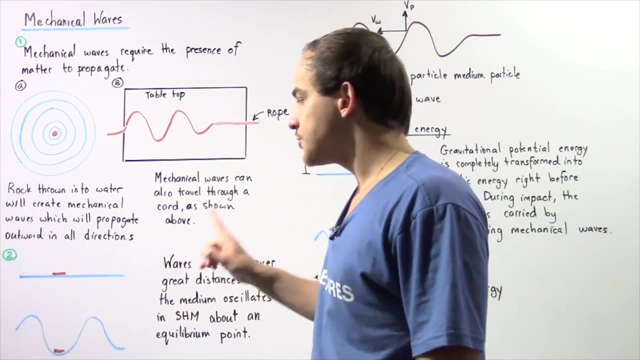 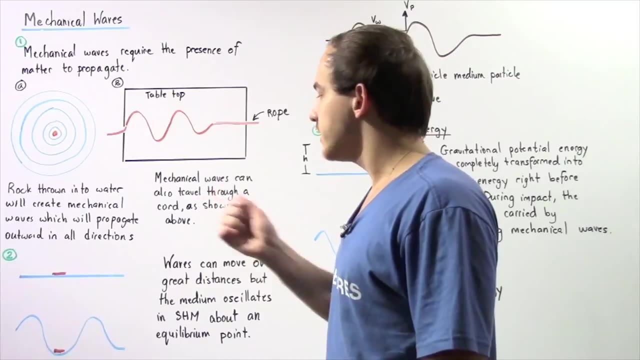 on the top of the water move along the following axis, or does it remain in the following position? Now, the answer is very important because it gives us an important property of waves. So when we're talking about mechanical waves, mechanical waves themselves can move over great. 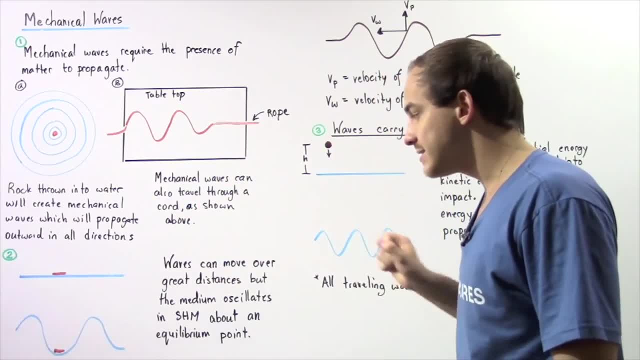 distances, but the actual medium oscillates in simple harmonic motion. a better way to explain it. So, when we're talking about mechanical waves, a better way to explain it. So, when we're talking about mechanical waves, a better way to explain it. 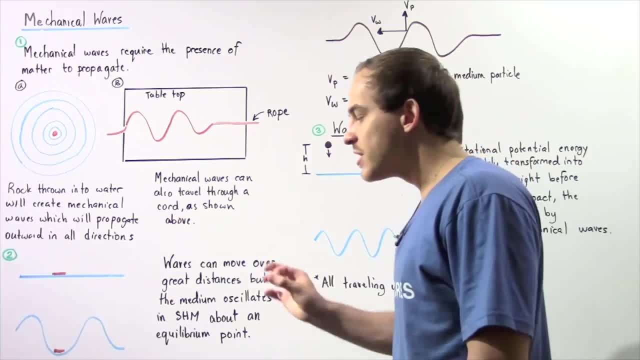 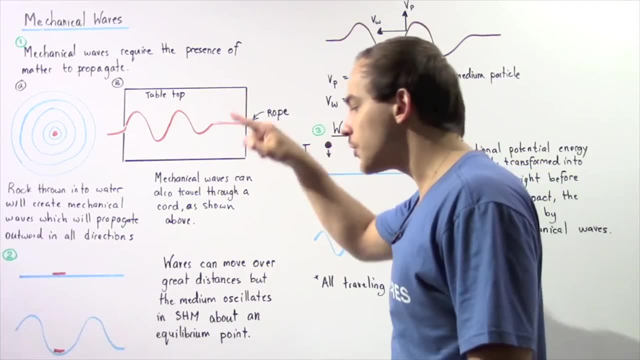 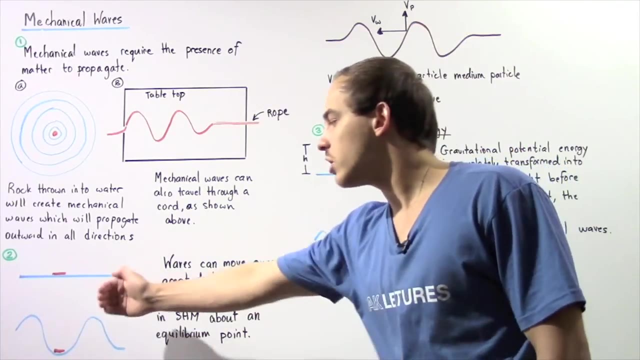 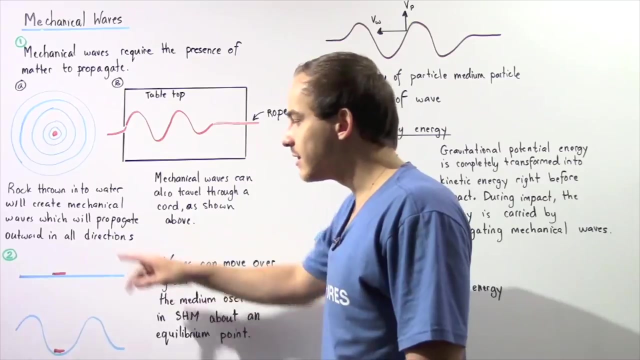 an equilibrium point. In other words, the individual molecules of the water oscillate back and forth about a vertical axis. Those molecules don't actually move along the following axis, along the horizontal axis, And that's exactly why, when I throw the rock and the water begins to oscillate, this leaf will remain in the following position. So it will. 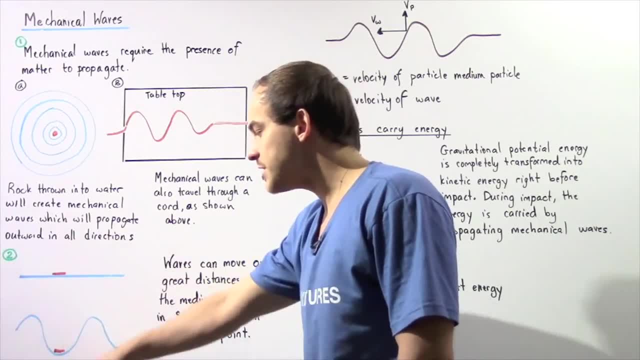 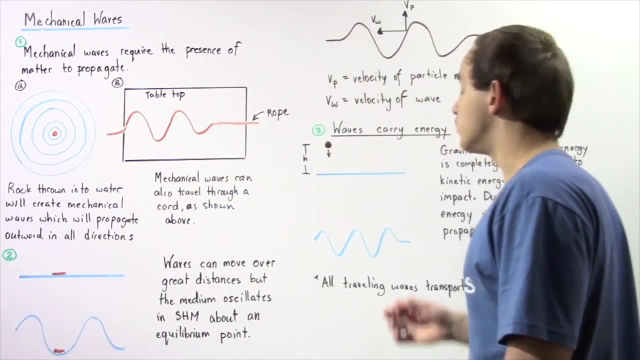 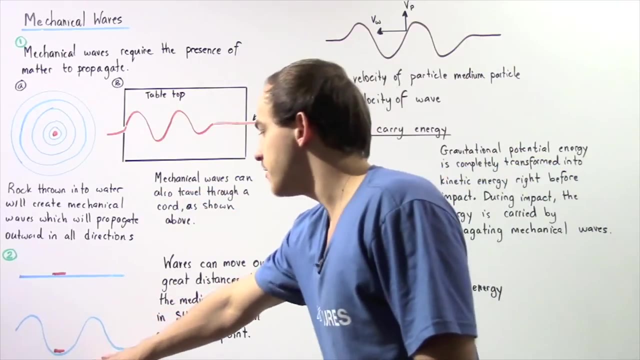 oscillate back and forth about an equilibrium position, but the leaf will not move along either direction, along our x-axis. So once again, the mechanical waves themselves propagate outward, for example in this case in the positive direction along the x-axis, but the individual 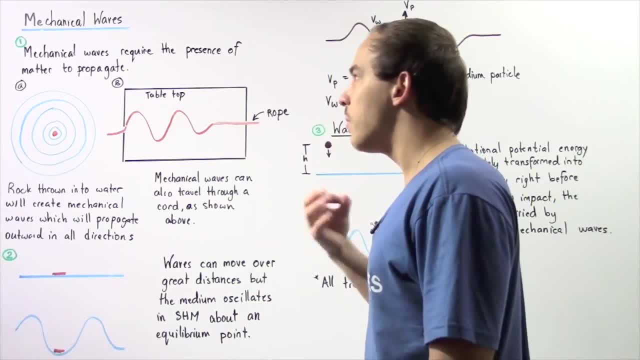 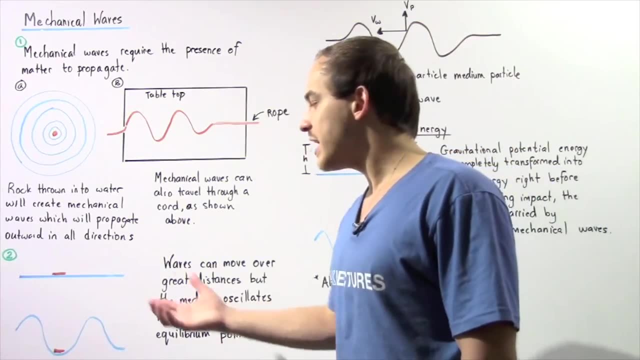 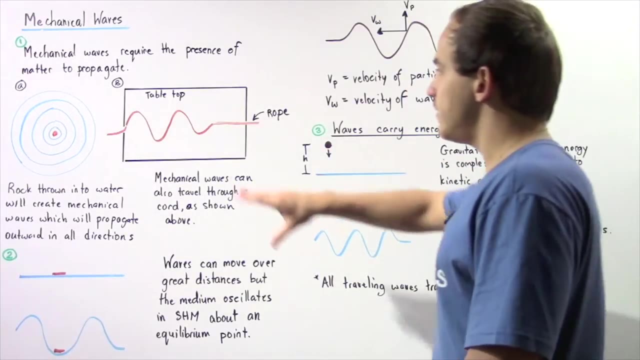 matter. molecules, the individual molecules composing our medium, don't actually move in the same direction that the wave moves. They oscillate about a vertical axis, about some equilibrium position. So, once again, if we look at example B, when we force our rope to propagate, 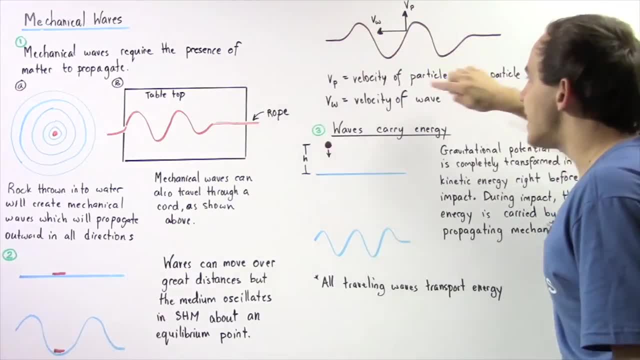 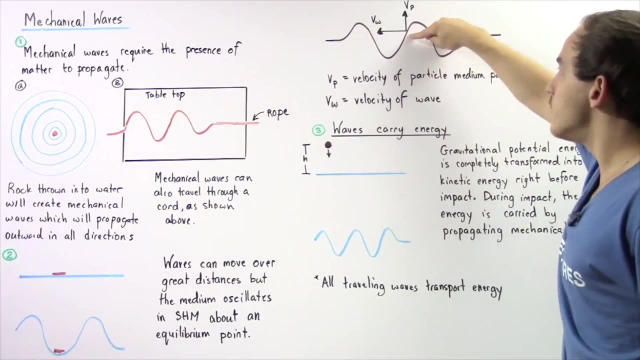 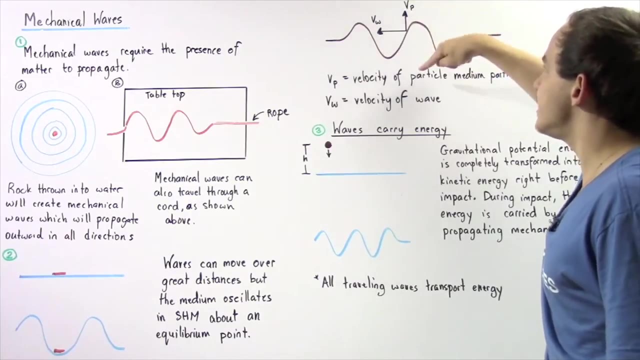 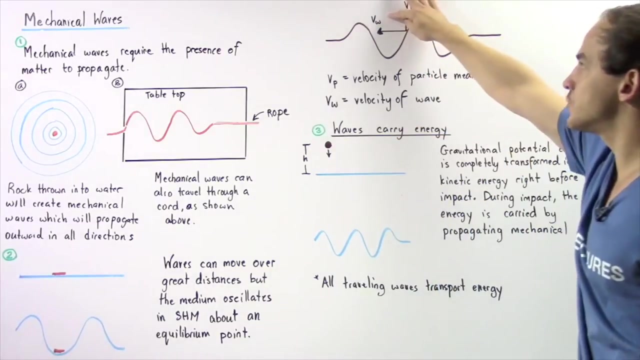 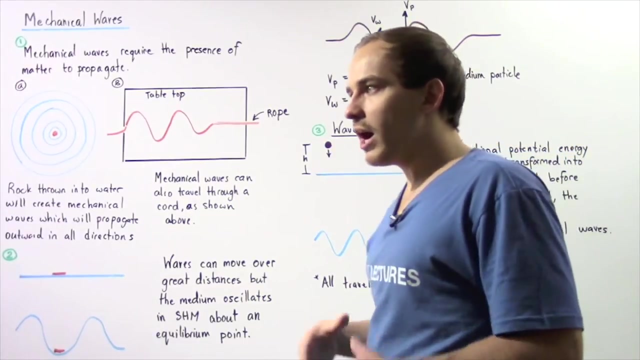 in the following direction. the actual velocity of the wave points in this direction, but the individual velocities of our individual particles composing our medium don't actually move in the same direction as the velocity of the wave itself. Now, what exactly is a wave? Well, a wave is. 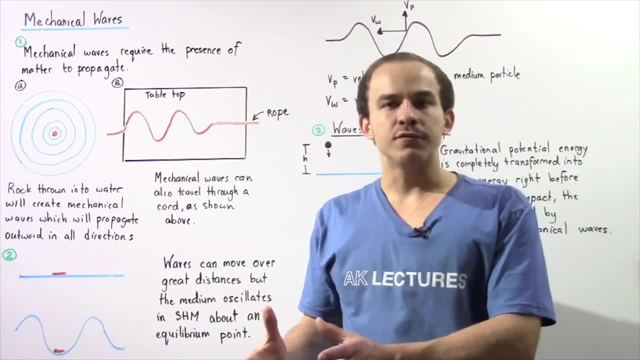 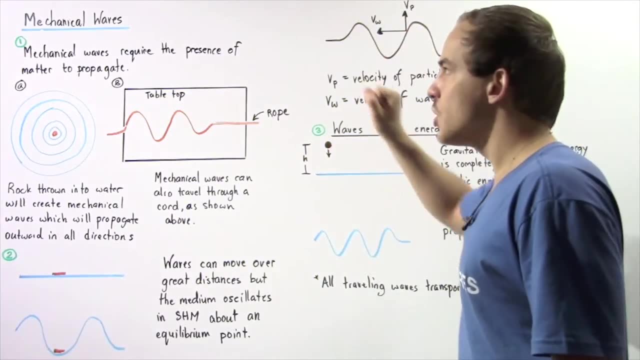 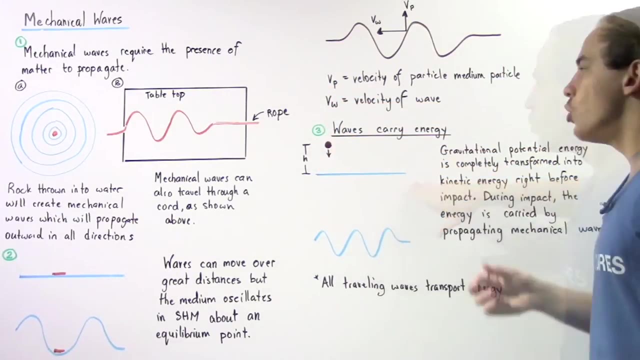 essentially one way that energy can be carried from one position to another position. So waves carry energy. So what happens when I force a wave to carry energy? Well, I force a wave to carry, I take my rock, I let go of my rock a certain distance h from the surface of the water. well, 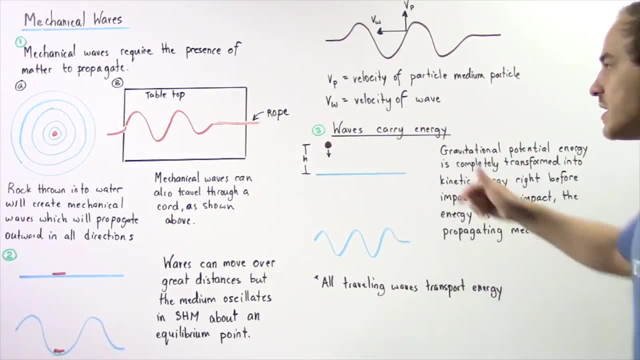 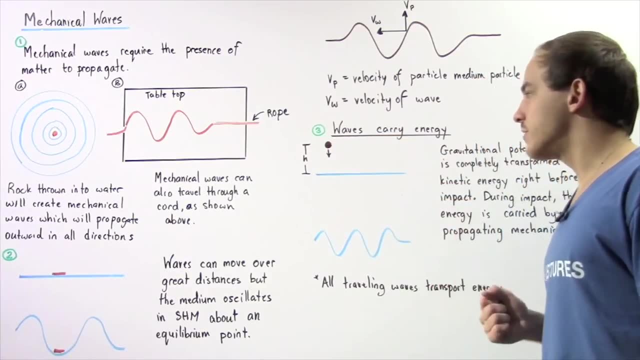 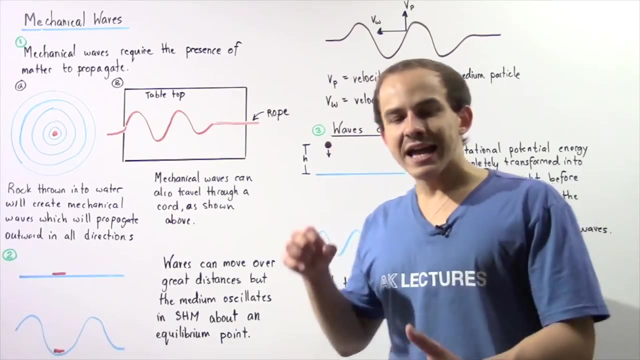 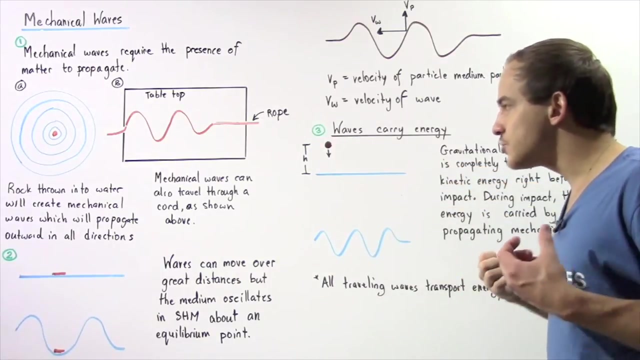 the rock initially has gravitational potential energy and as it travels downward it gains kinetic energy, and right before it impacts the surface of the water, all that gravitational potential energy has been converted to kinetic energy, and when the object makes impact, when the object hits the surface of the water, that energy is transferred to the molecules of the water.